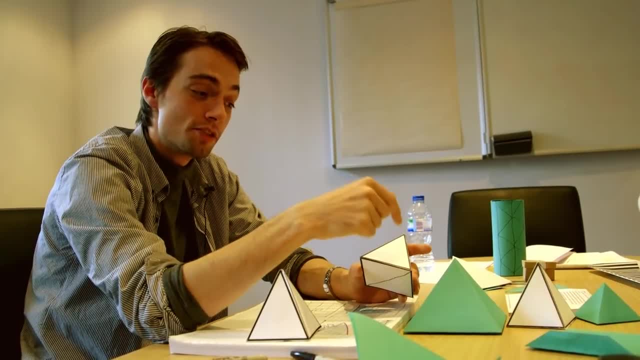 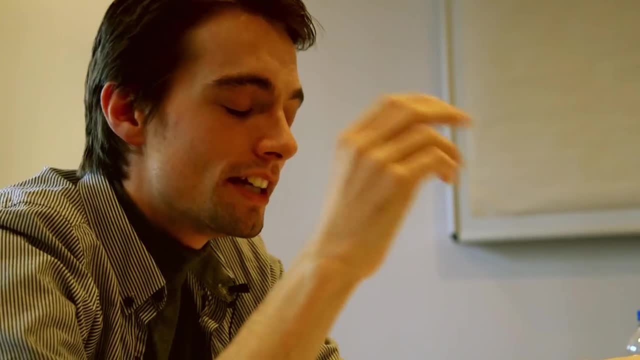 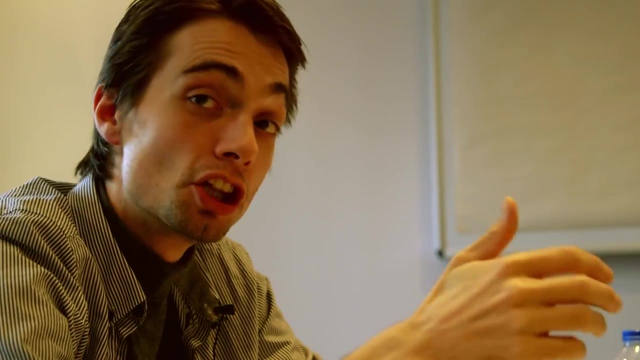 With all of these inputs we can finally generate a shaded value to say: well, this is well lit, or it's facing away from the light, so it's in shade, and so on and so forth. The equations that we do, the computation of the light value at every pixel is local. 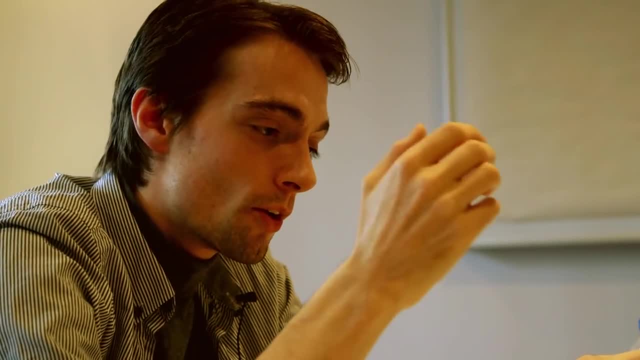 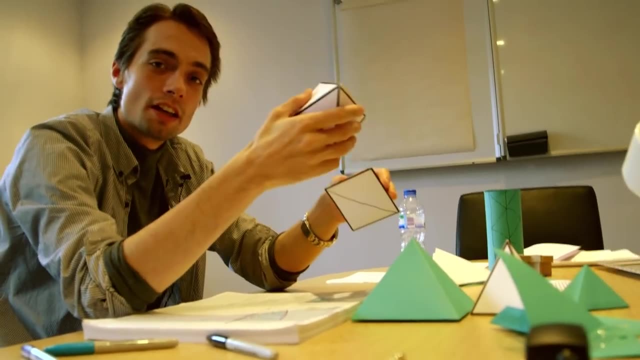 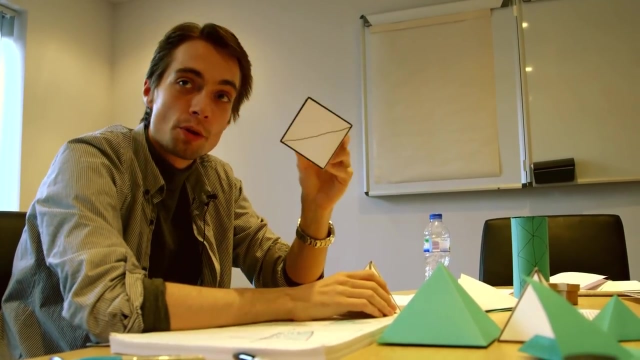 It's local, to the surface that we're lighting, Because in all of our work that we've done getting down to pixels, we're not really holding on to any other information about the rest of the scene. We only know about the one object that we're working with at a time. 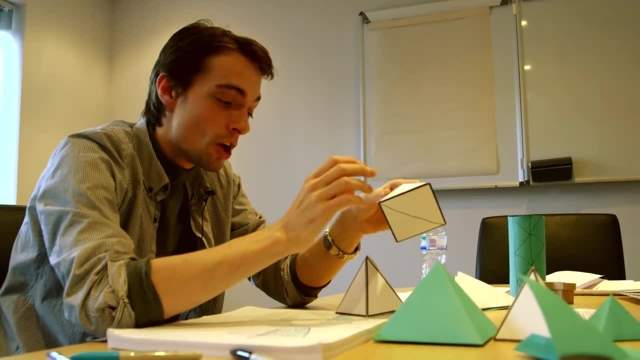 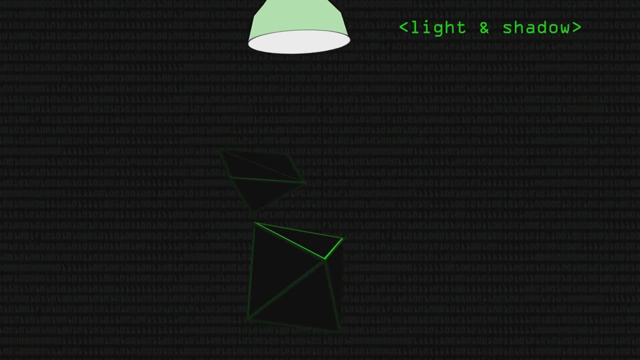 So we only know about the pixels on the surface of this object. We don't know, for example, if there is another object here blocking the light reaching this object. So we can't know, So we can't account for that in our simple light model at this pixel. 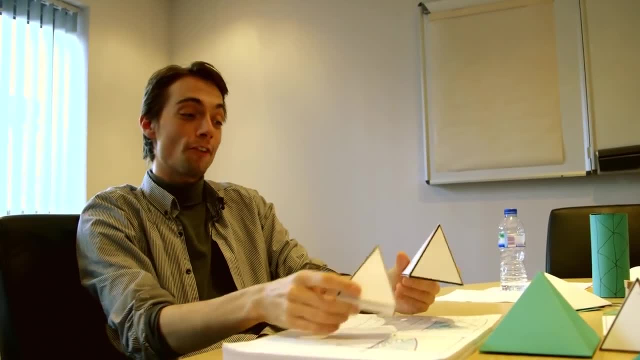 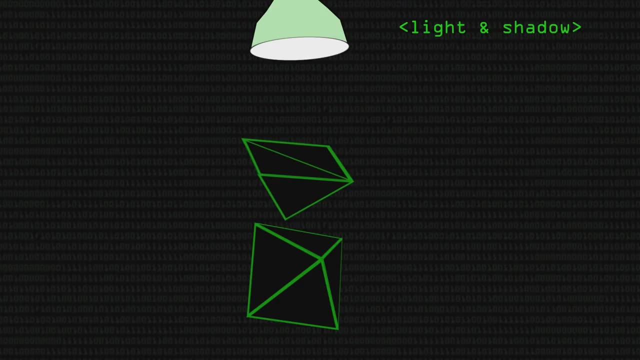 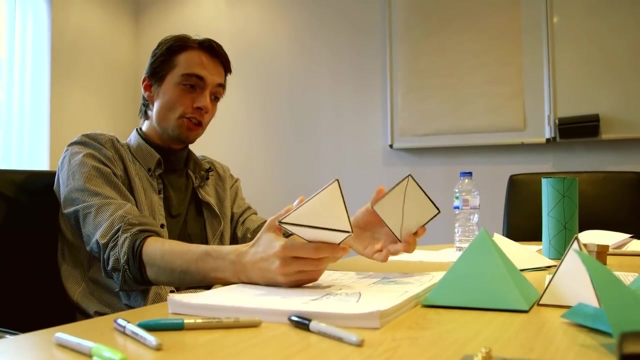 So in older computer graphics, when you look at them, you'll often see that actually you can see these local light models in action, and the lack of shadows is quite apparent. How then do we get that information? How do we get that global information to augment our local light model and, for example, render shadows? 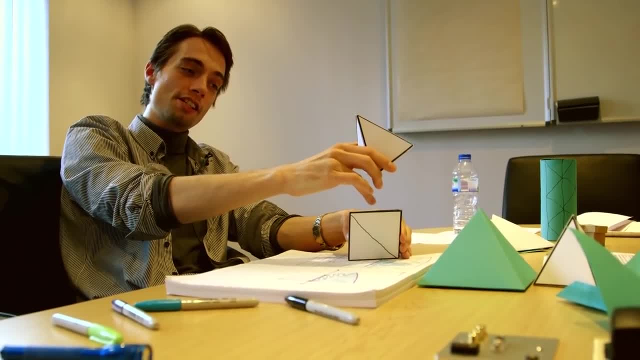 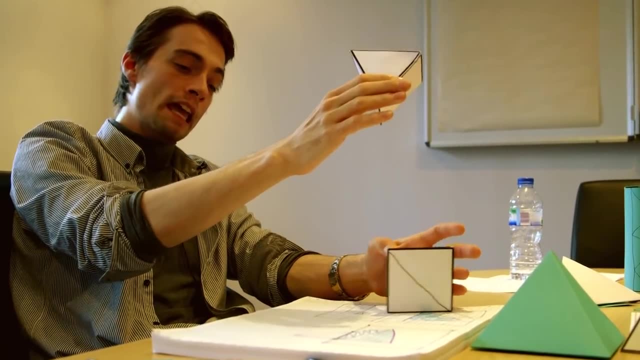 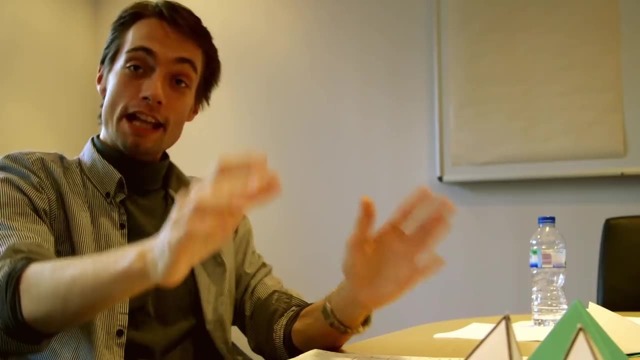 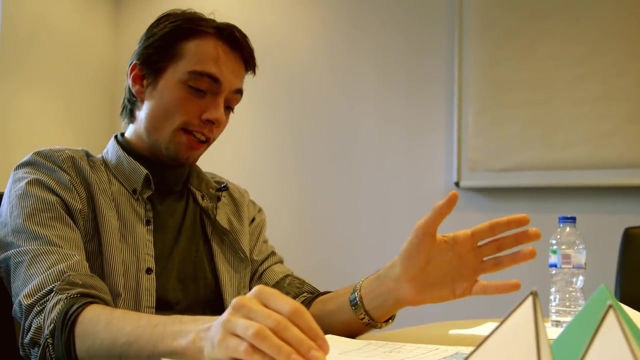 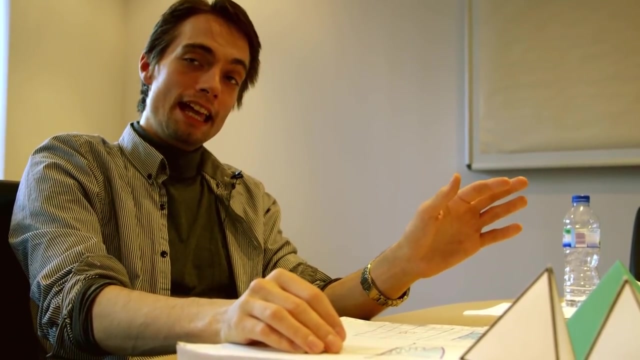 How do we decide that this point on the surface Is being occluded by another object somewhere else in the scene? And the answer to that, or one solution, is to go back to our friend, the depth buffer. The depth buffer, as we'll remember, is a representation, at every pixel, of the depth of that pixel in the scene. 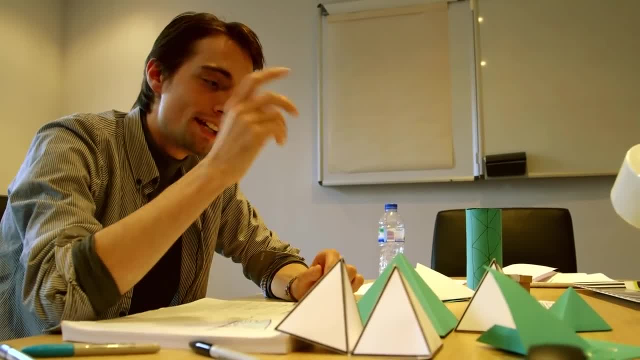 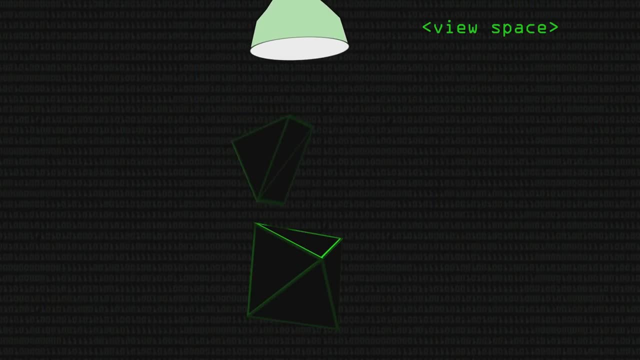 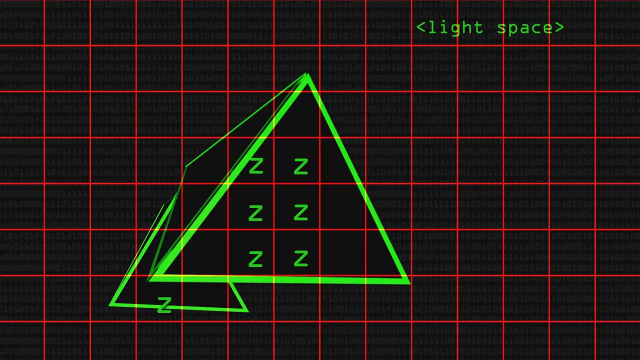 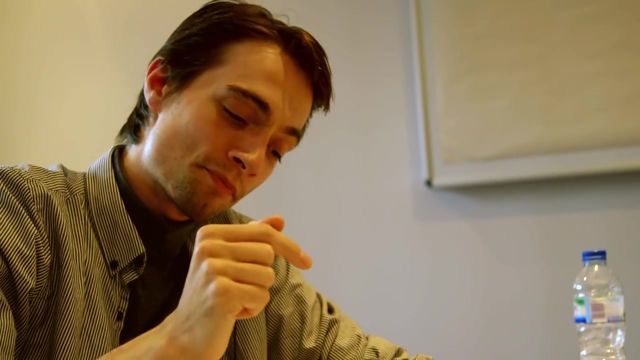 What we can do is we can render the scene not from the camera's point of view, but from the point of view of the light. Rather than rendering shaded pixels, however, we just output the depth buffer values. So what we end up with is a buffer of data containing the depth per pixel: depth from the position of the light. 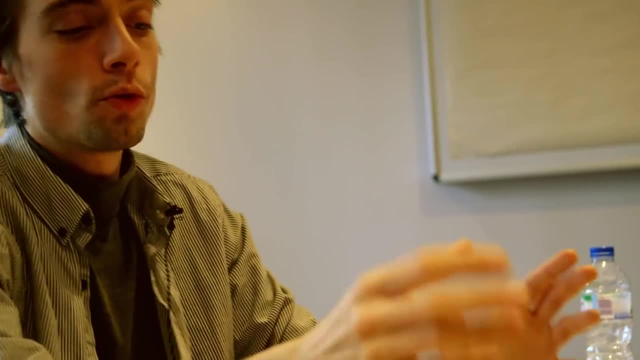 So what we end up with is a buffer of data containing the depth per pixel depth from the position of the light. Why is that a useful thing to have? Well, what we've done really is: we've rephrased the question. 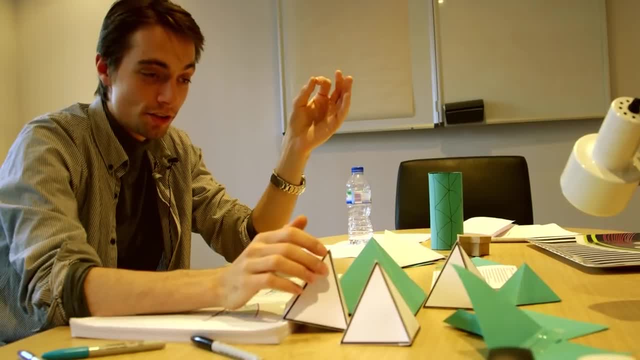 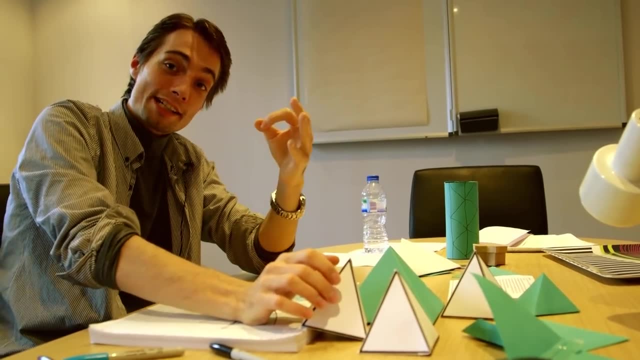 We're not saying: is such a pixel in light or shade. We're saying: is such a pixel visible to the light? Because if a pixel is visible to the light, then it's being illuminated. If it's not visible to the light, then it's in shadow. 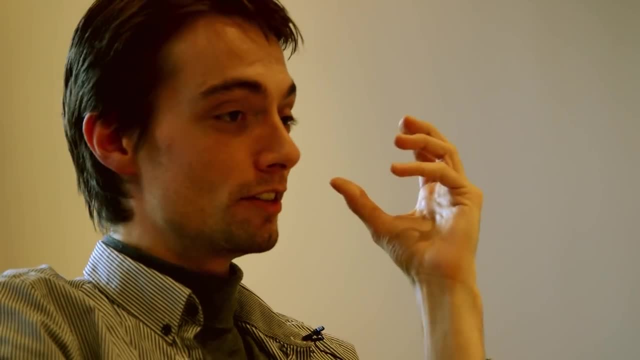 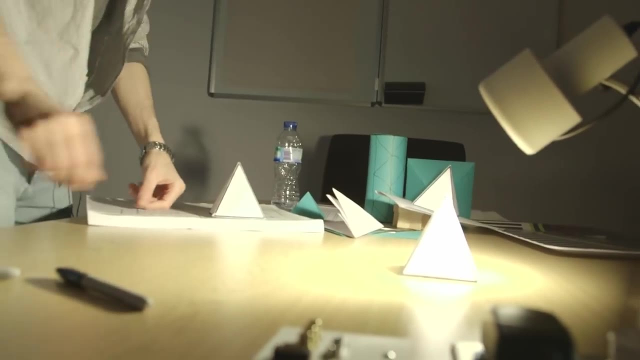 It will probably be clearer to actually cast some shadows into this. It will probably be clearer to actually cast some shadows into this. There we go. Did we get a good shadow on that? Oh no, not really. That's a bit better, isn't it? 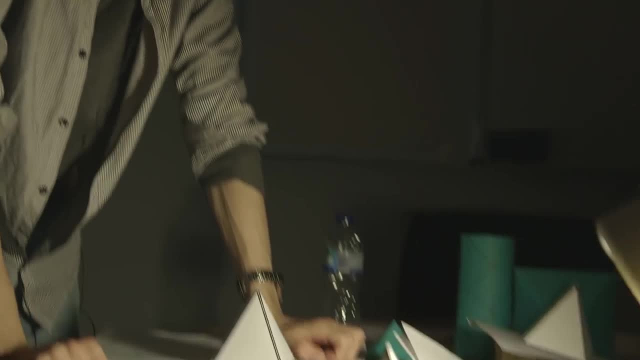 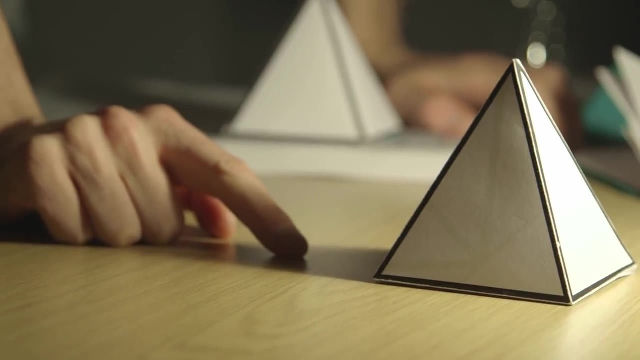 Right. So we have our scene, a simple pyramid. We'll incorporate the table into this because this is where the shadow is being cast. So the table is another 3D object in our 3D world and we want to shade a point here. 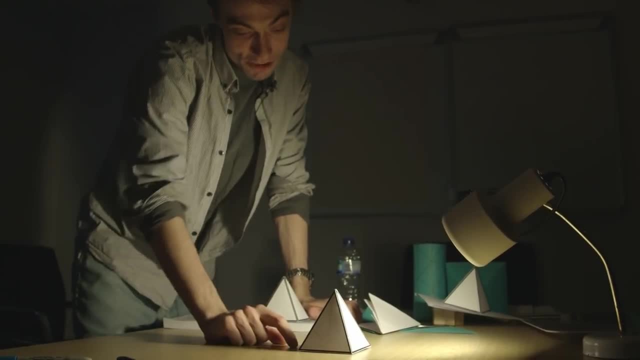 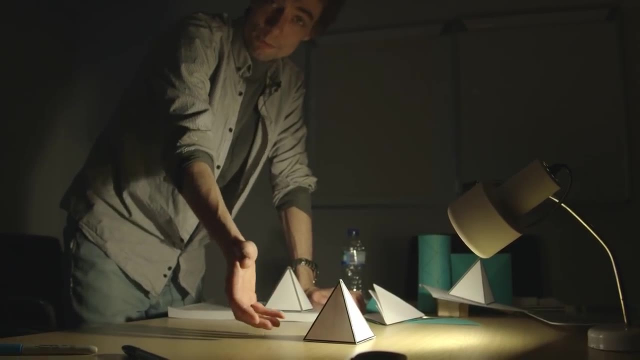 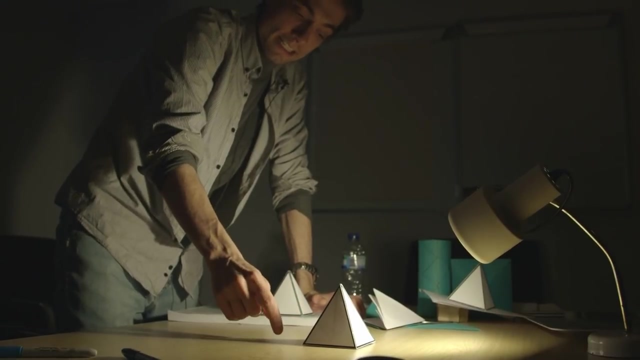 So for that, not only do we need to know properties of the surface- at this point, the normal and the, the material properties and the direction of the light, and so on and so forth, but we also want to know whether it's in light or in shade. 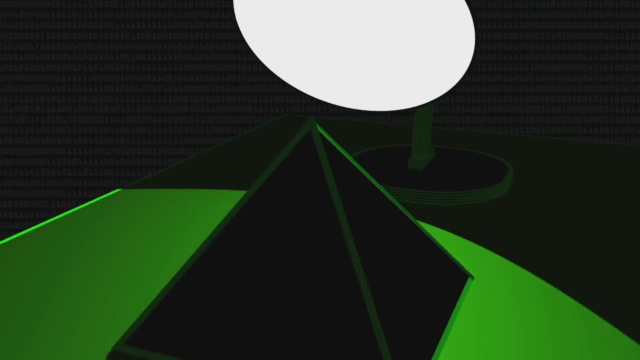 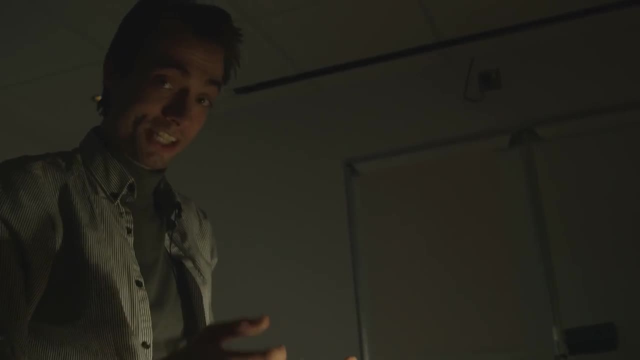 So how do we determine that The shading of a pixel is local and we don't have information about the rest of the scene, So we can't know whether or not a certain point is being occluded by another object in the scene. We don't know whether it's in shadow or not. 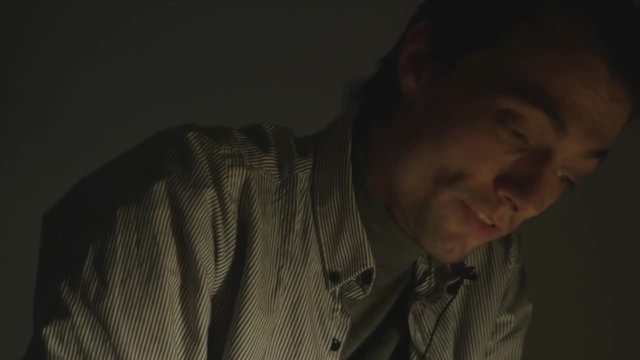 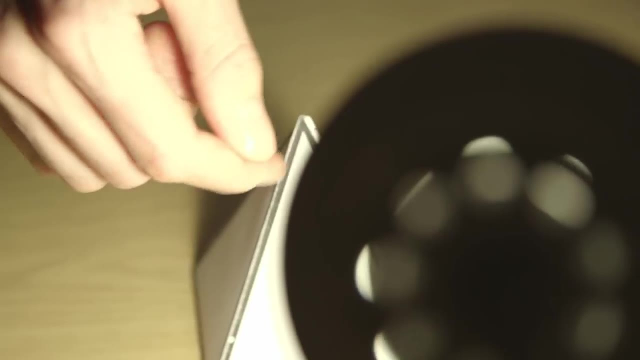 To solve that problem, we use a two-step process That involves the Z buffer. First of all, though, we render the scene from the point of view not of the camera, but of the light. What we do is we record not colour information, but depth information. 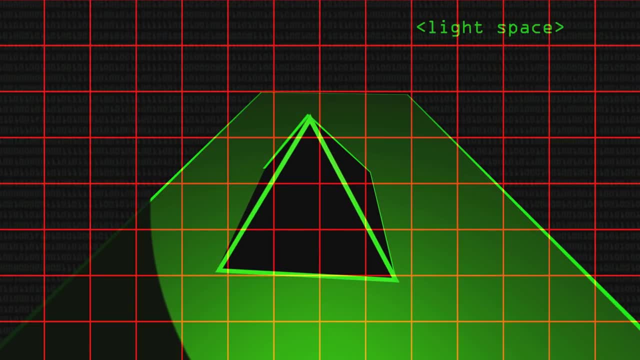 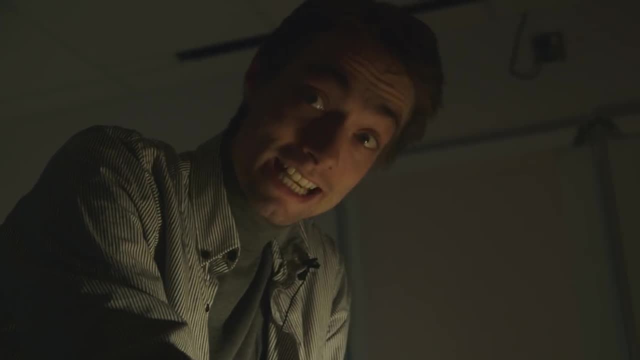 exactly as we would do in normal rendering, In other words, we render into the depth buffer and we record at every pixel exactly how far away every pixel is from the point of view of the light And we save that information in a buffer for use later. Then, when we come to render the scene from the point of view of the camera, we take this point here and we project it out of world space, where it is, into light space. So what we know, then, is exactly how far away the point that we're shading is. 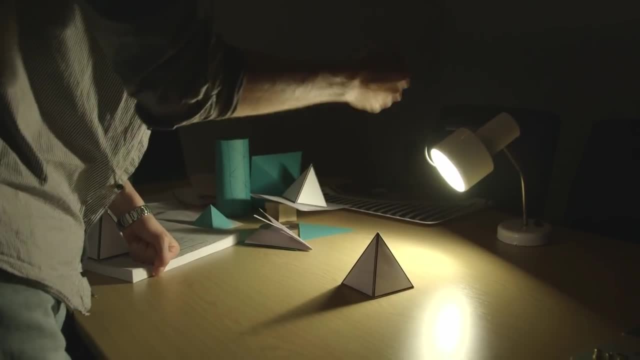 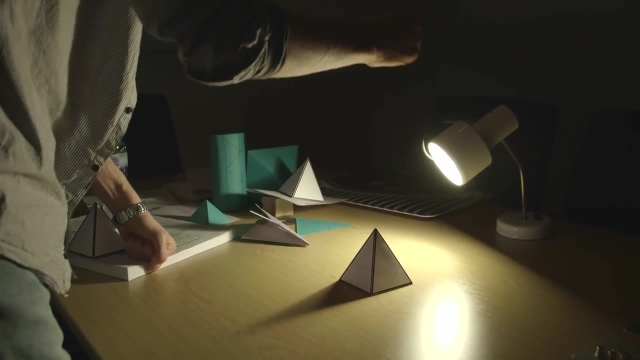 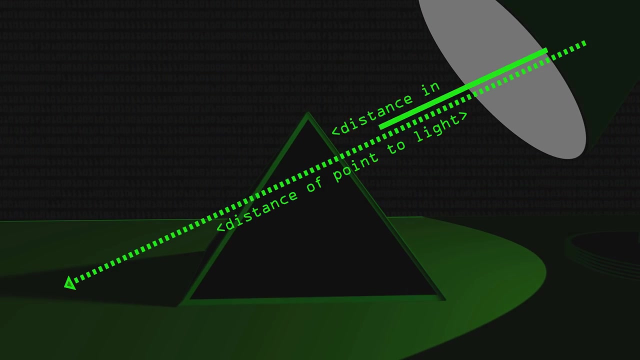 from the point of view of the light. What we can then do is do a lookup into the Z buffer from the light pass that we rendered before, And we can find out how far away that point is from the light and compare it to the value in the Z buffer. 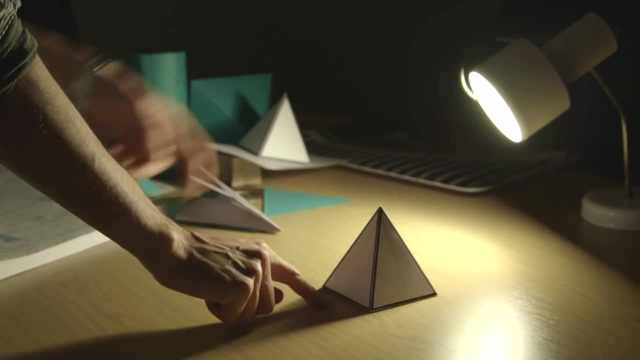 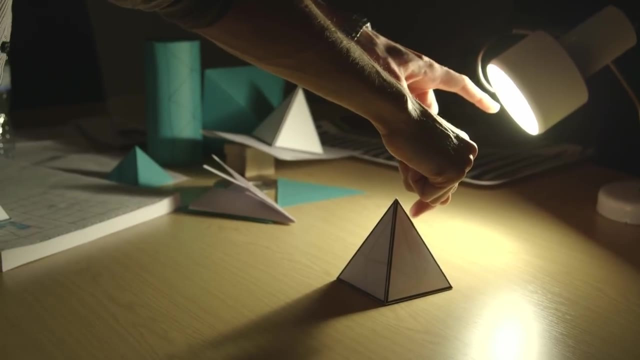 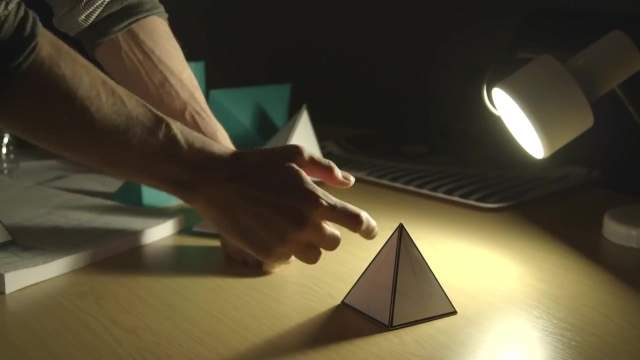 So in this case we find that the depth from the light at this point is further than the depth from the front face of the pyramid here. Therefore, it's in shadow And we don't need to do our lighting here or we need to incorporate that information into our lighting equations. 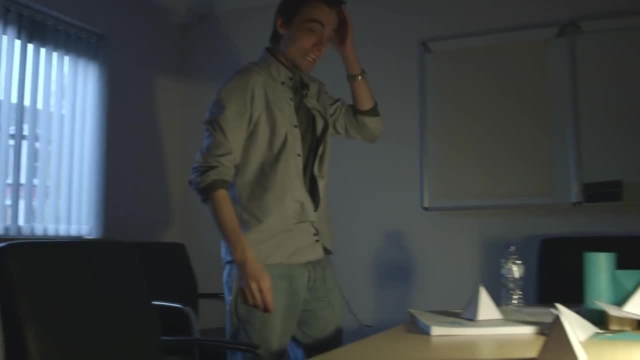 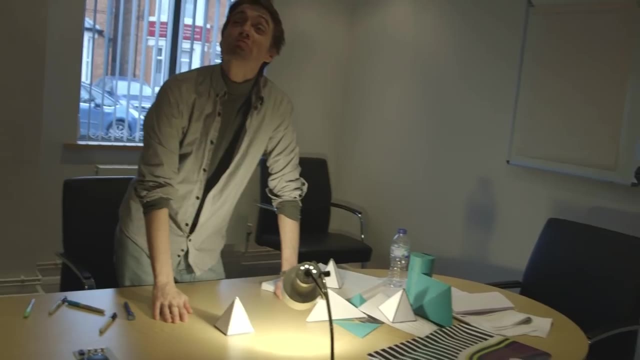 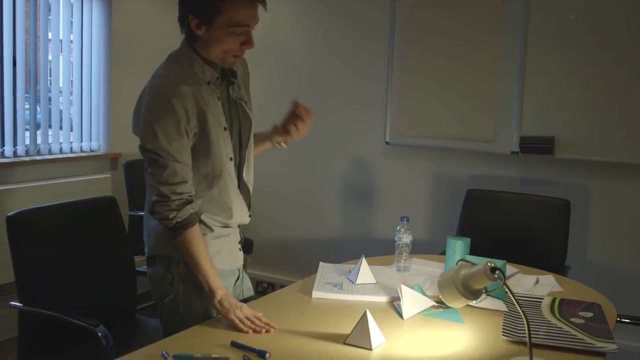 So if we add another light, that's not done anything at all, But in theory we can have as many lights as we like. Plenty anyway, yeah. So in theory we can have as many lights as we like, as long as we are prepared to render the scene again and again. 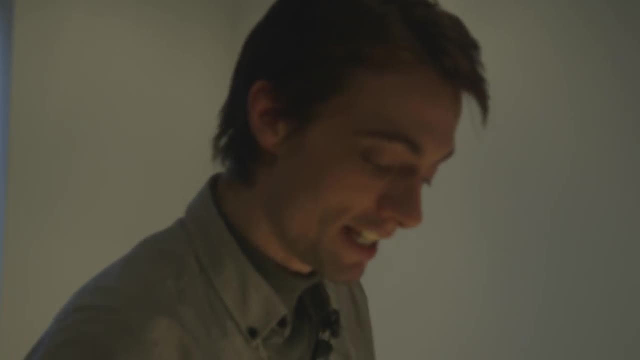 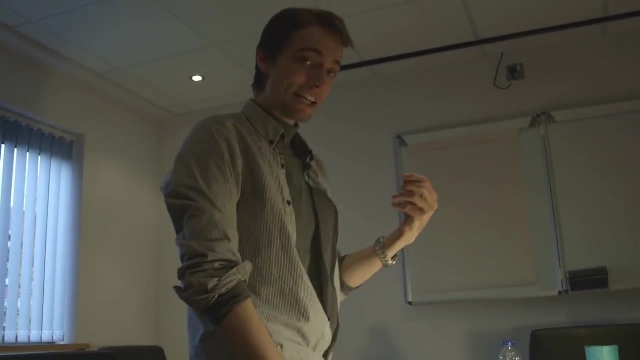 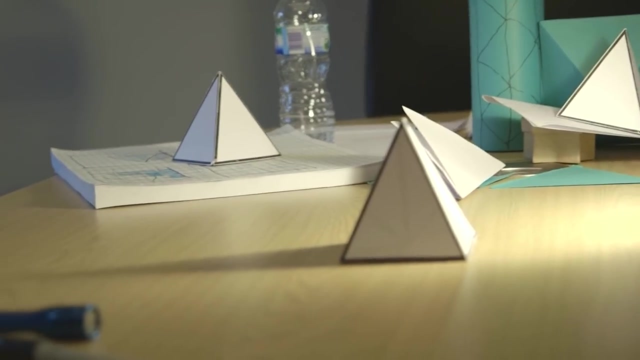 from the point of view of every light, so that we have enough information when we come to shade in the pixels to be able to do that lookup and say, is this still in shadow from this particular light or is it being illuminated? And in modern games and things like that. 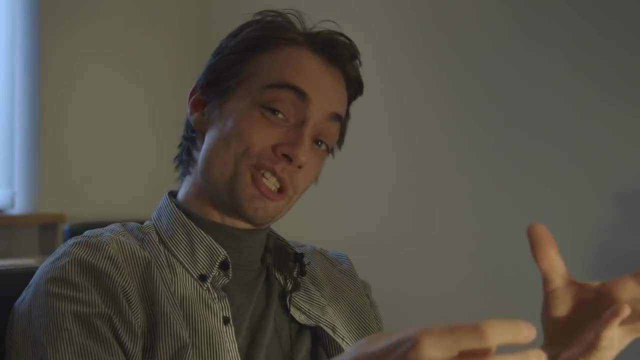 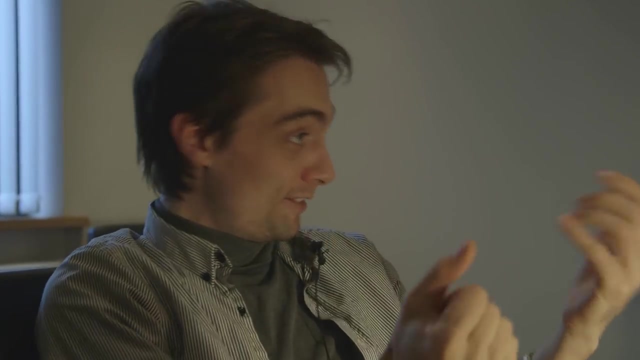 now we can have multiple lights because we can afford to render the scene multiple times from multiple perspectives in order to build up that information. However, if you look back just maybe 10 or 15 years at older games and things like that, you tend only to have one shadow casting light. 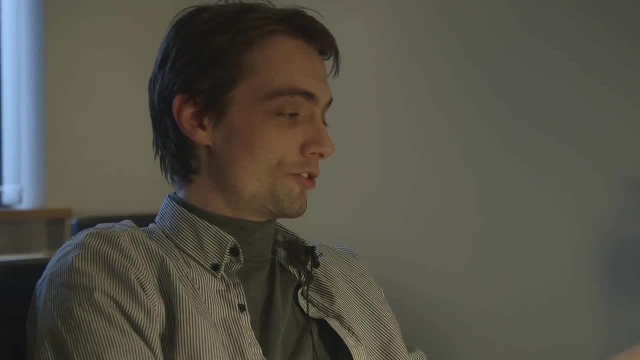 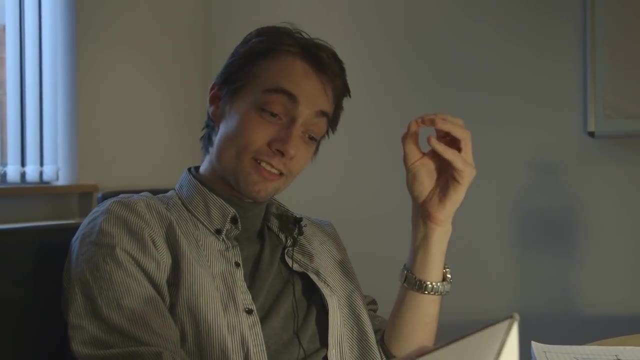 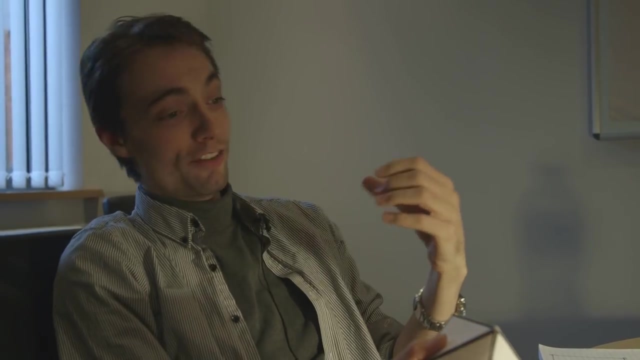 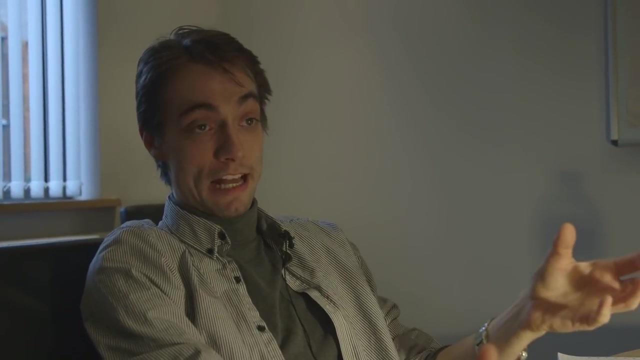 or maybe not even any at all, because rendering hundreds of thousands of of triangles every single frame is expensive in terms of time, And so it's sometimes better just to accept the quality loss and not have any shadows rather than go for complete realism, And often, naturally, you find that a single shadow 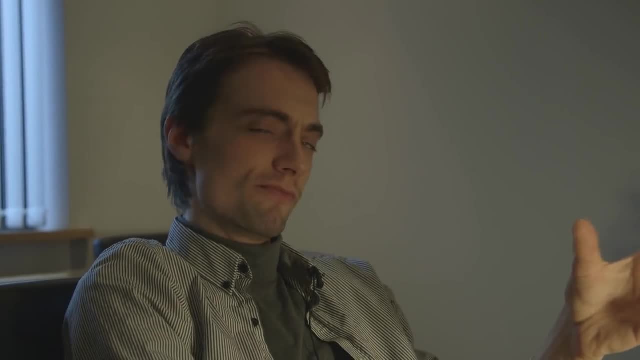 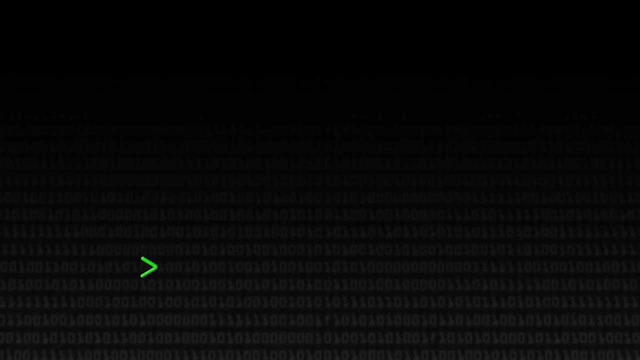 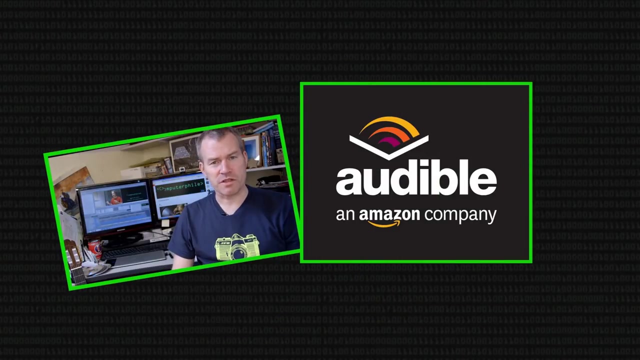 looks much better than no shadows at all. but two or three shadows only looks marginally better than one shadow. So it is a law of diminishing returns. It is a law of diminishing returns. We'd like to thank Audiblecom for their support of this Computerphile video. 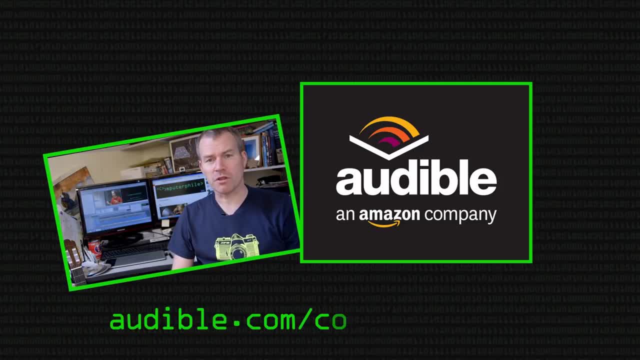 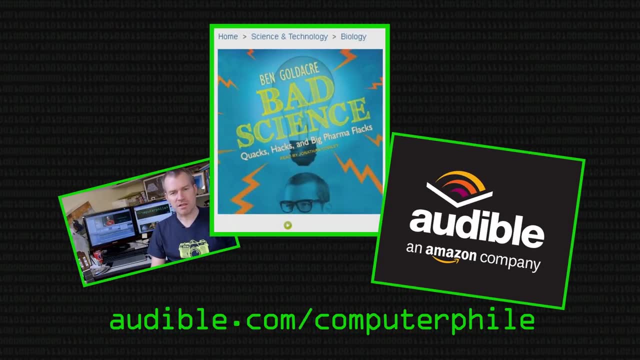 and if you'd like to download one of their huge range of books, go to audiblecom, slash computerphile and you can sign up and download one for free. I'd like to recommend a book called Bad Science by Ben Goldacre, and for those of you interested in science, it's fantastic.